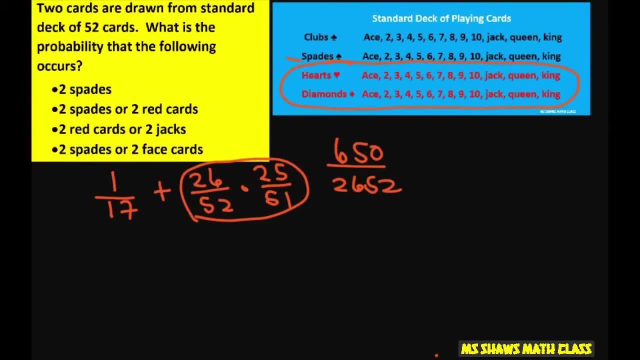 You just put in the calculator. This reduces to one divided by 17, plus 25 divided by 102.. And that's, That's going to end up being 31 divided by 1, 0, 2.. All right, Now two red cards, which we already know what that is. 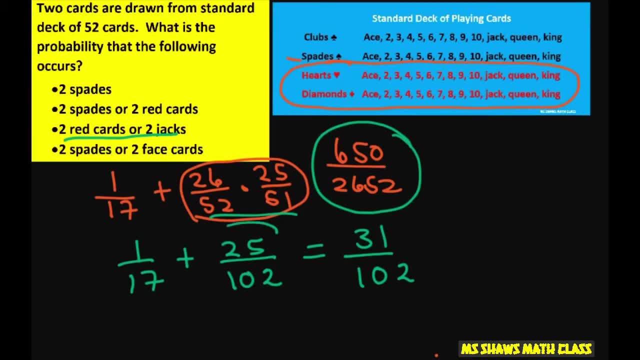 the two red cards. that reduces to 25 divided by 102.. So the two red cards is I just forgot and I just said 25 divided by 102, or two jacks. So the jacks, we have four jacks. 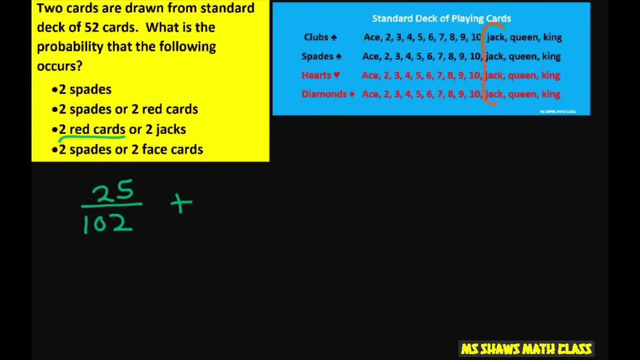 So let's do the four jacks- Four out of 52. Times three, Three out of 51, because you don't replace it. However, we already counted the two red jacks into this first part, because we already counted our red cards. 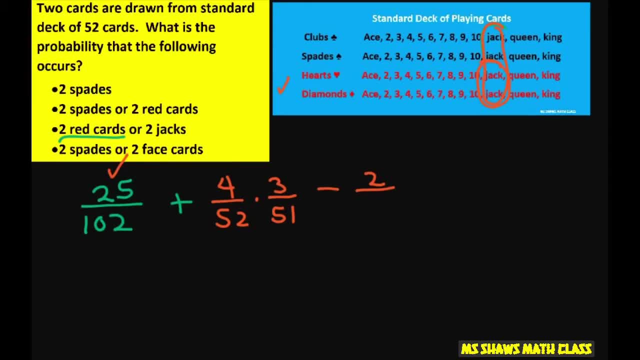 So we're going to have to subtract two divided by 52, times one divided by 51. You have to subtract that out, So I have 25 divided by 102.. Plus 12, minus two divided by two, what's this number? 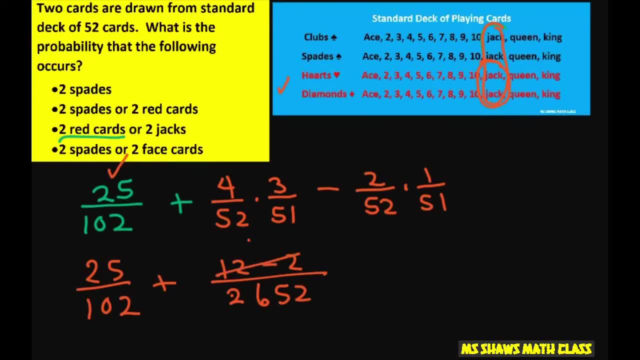 Six five two. Again, you could just use your calculator. That's going to change to 10.. And then it makes it easier to put in the calculator if you simplify first. So that's going to end up being 55 divided by 221.. 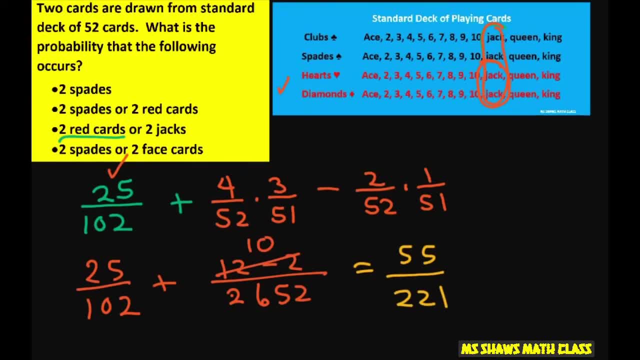 And the last one, We have two spades. we already know that one, two spades is one divided by 17, plus the two face cards. So face cards are these and there's a total of 12.. So that's going to be 12 divided by 52, times 11, divided by 52.